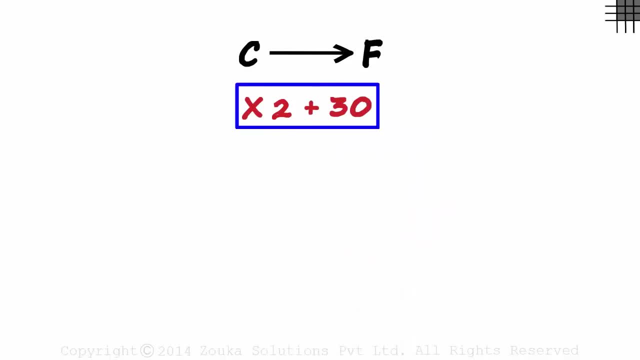 and add 30 to it. That will give us the answer. in Fahrenheit, Say 10 degrees Celsius. We need to convert this into Fahrenheit. Multiply it with 2 and add 30.. 20 plus 30 is 50 degrees. 10 degrees Celsius is approximately 50 degrees Fahrenheit. 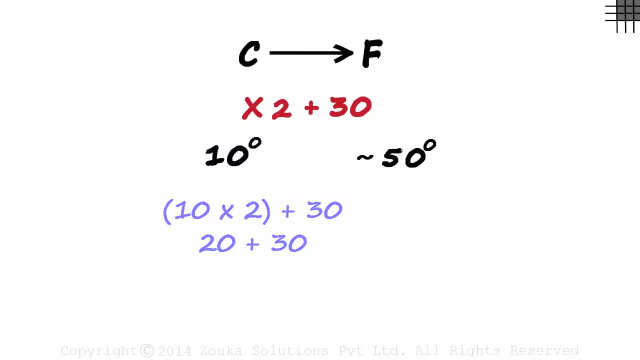 Multiply with 2 and add 30 to the product 17 degrees Celsius. 17 times 2 is 34.. And 34 plus 30, is 64.. 17 degrees Celsius is approximately 64 degrees Fahrenheit If we do the exact calculations using the formulae. we would have got 10 degrees Celsius as 50 degrees Fahrenheit- Yes, we were a bit fortunate here- And 17 degrees Celsius as 62.6 degrees Fahrenheit- Almost equal. The higher the temperature, the bigger will be the difference. Say 50 degrees Celsius, 100 plus 30 is 130 degrees Fahrenheit. The exact answer is 122, a difference of 8 degrees Fahrenheit. And converting 100 degrees Celsius to Fahrenheit, we get 230 degrees approximately, And the exact answer is 212 degrees Fahrenheit. 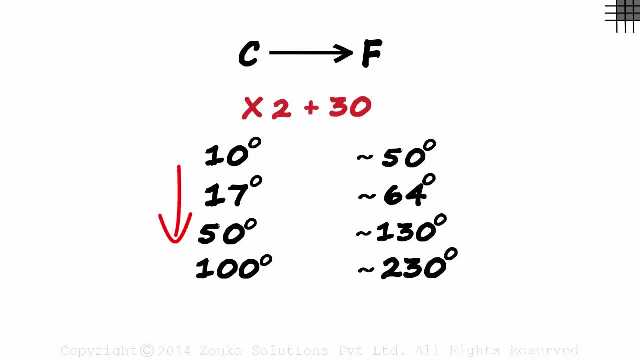 So as the number increases, the difference or error in the answer also increases. Does this work for negative temperatures as well? Absolutely Say: minus 15 degrees Celsius, Minus 15 times 2 is minus 30. And minus 30 plus 30 equals zero. 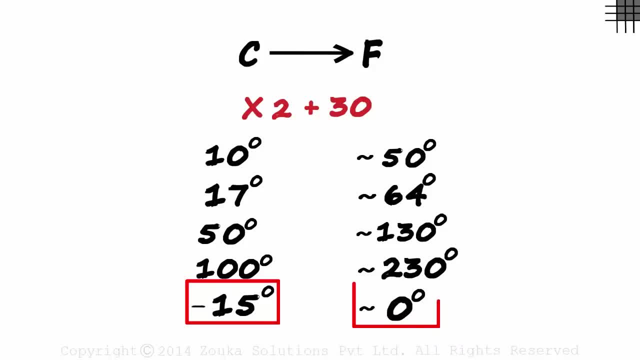 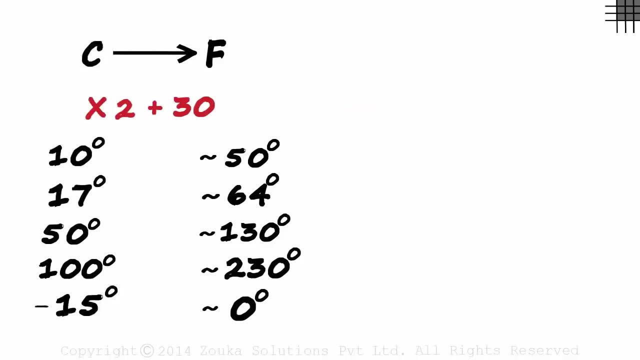 Minus 15 degrees Celsius is approximately zero degrees Fahrenheit. The exact value comes out to be 5 degrees Fahrenheit. So to convert from Celsius to Fahrenheit, just multiply by 2 and add 30 to the product. And how do we quickly convert Fahrenheit to Celsius? 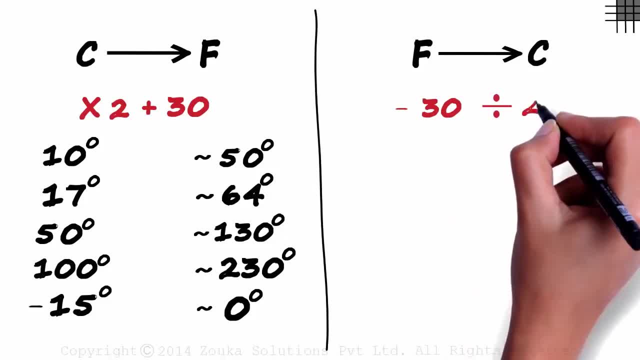 Easy. We subtract 30 and then divide by 2.. Take 100 degrees Fahrenheit, for example. We subtract 30 and get 70. And 70 over 2 is equal to 35.. 100 degrees Fahrenheit is approximately equal to 35 degrees Celsius. 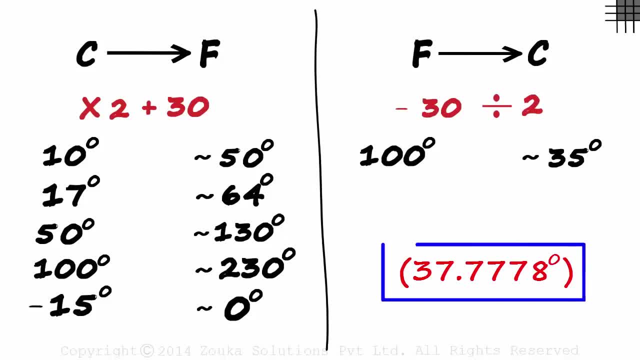 The exact answer, if you calculate, is 37.7778 degrees Celsius. The difference isn't much. What about 72 degrees Fahrenheit Subtract 30 and get 42.. 42 over 2 is 21.. 72 degrees Fahrenheit is approximately equal to 21 degrees Celsius.